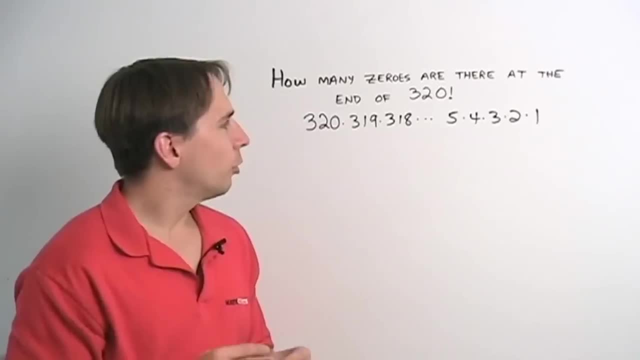 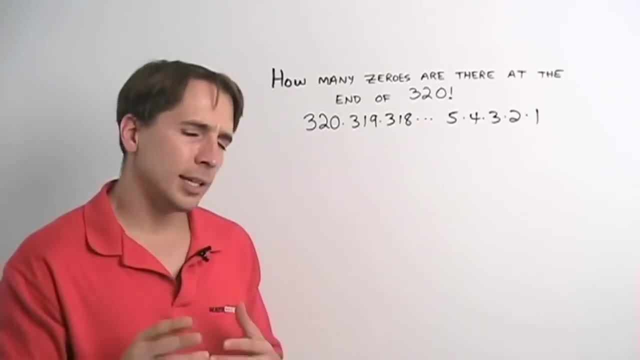 this amazing talent for multiplying out huge products. So a group of students. we offered him $20 to multiply out 100 factorial with a pencil and paper. So he sat down and started multiplying out the numbers. Then, after about 25 minutes, some of the instructors found 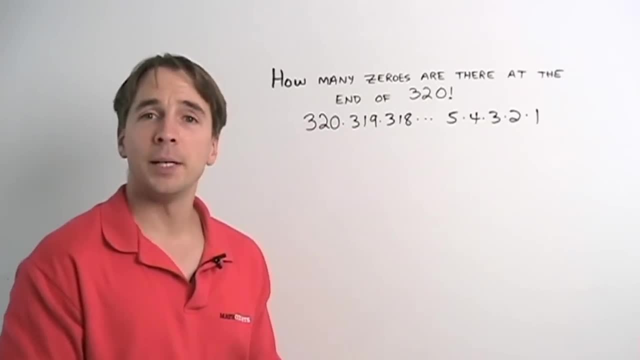 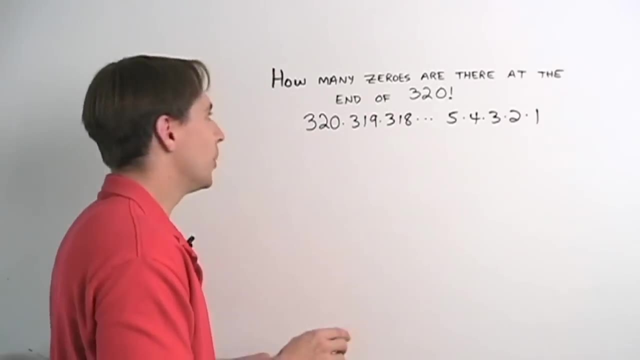 out what was going on, And they came over and paid him $20 to stop. at which point, well the rest of us? well, we started out multiplying out 100 factorial, hoping they'd pay us to stop too. That didn't work and this probably isn't going to work for us in. 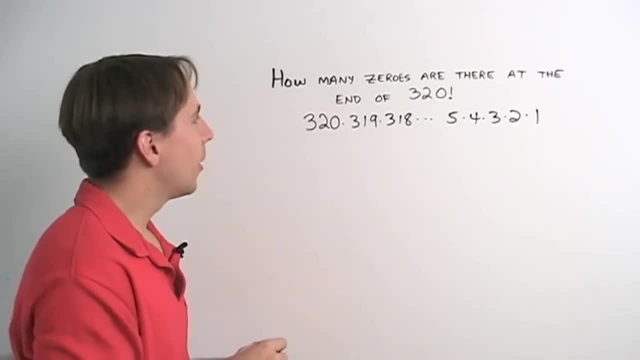 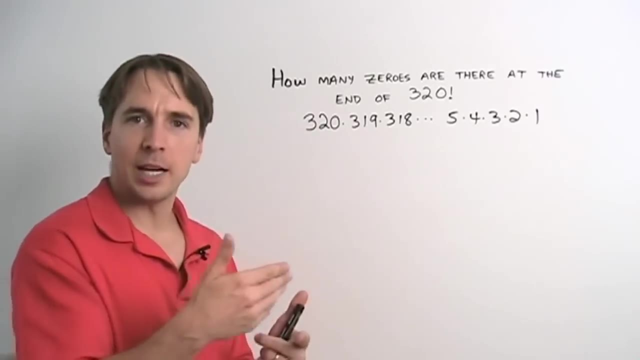 solving this problem. So we're going to have to think a little bit harder about this. Zeros at the end of numbers. How does that happen? Well, that happens when you multiply by 10.. 14 times 10,, you get 140 zero at the end. So you think, well, let's just count. 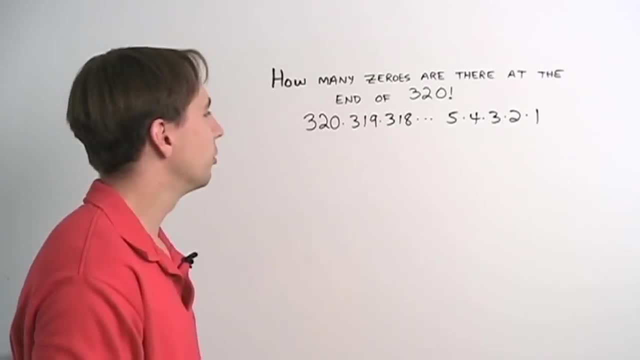 up the multiples of 10.. There's 10, there's 20,, 30,, 40, and up to 320.. So obviously there are 32 of these multiples of 10.. So maybe there are just 32.. 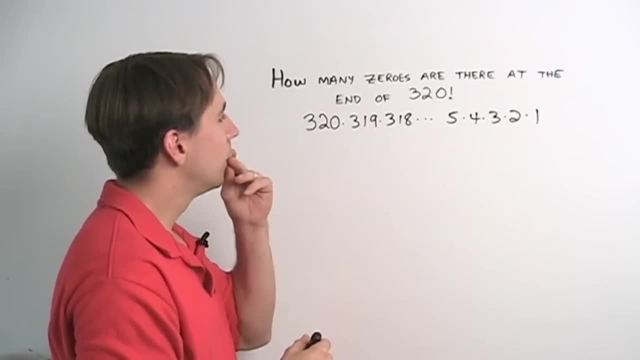 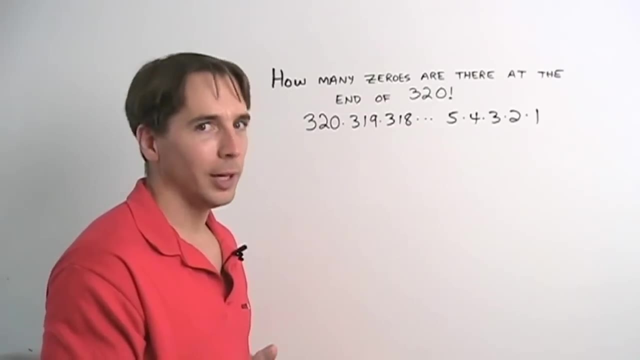 There are 32 zeros and 325.. Oh, but wait a second, I see there's 5 and a 2.. And when we multiply 5 and 2, well, any time you take a 5 and a 2 and you multiply them, you get. 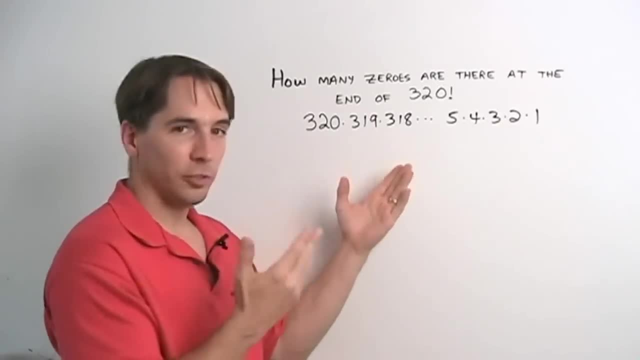 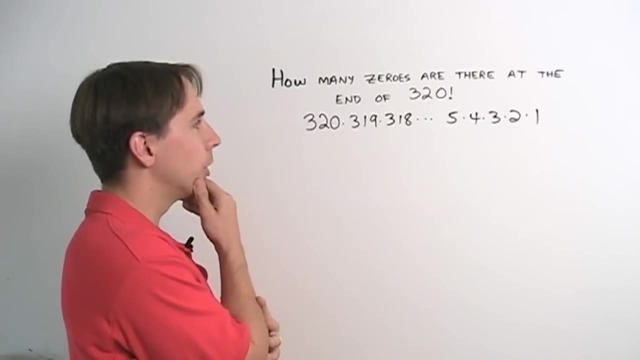 a 10, and that's going to give us another zero, And then there's 15.. Same thing's going to happen. I'm going to end up multiplying that by some even number, get another 10, and, oh boy, back to the drawing board. 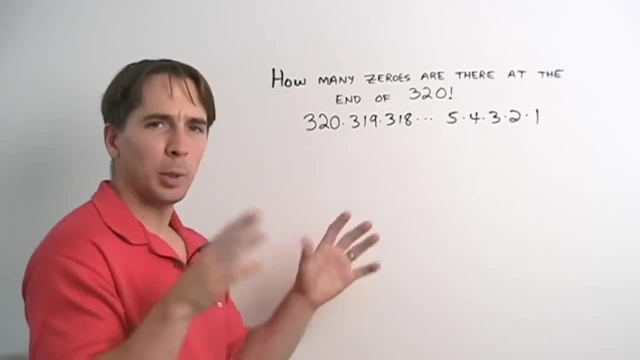 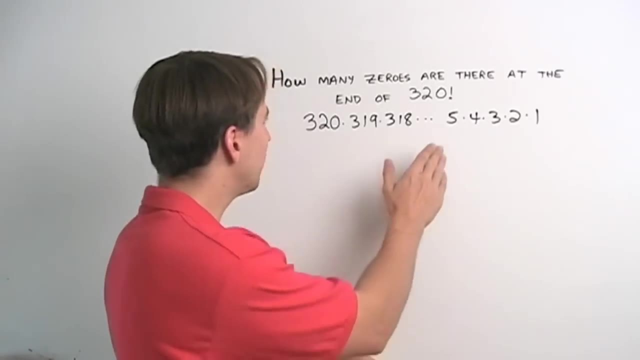 Looks like what we need to worry about are the 2s and the 5s. Now they're probably going to be way, way more than that, So let's just think about the 5s first. Maybe, if we can count how many 5s, how many factors. 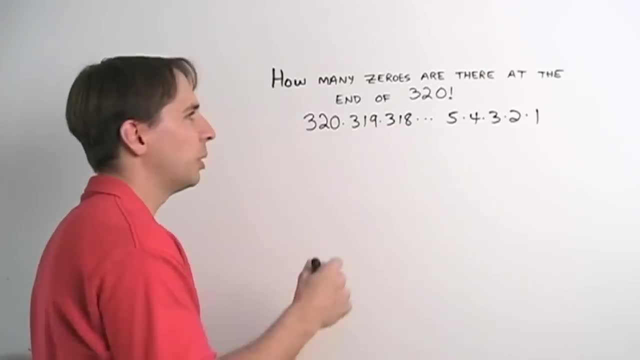 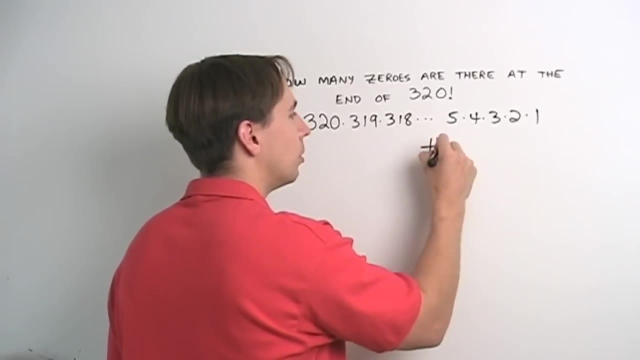 of 5 there are here. well then, we can just pair them up with 2s and make 10s. So we'll start by counting up the multiples of 5 in this list, Number 5s, let's see. Well, if 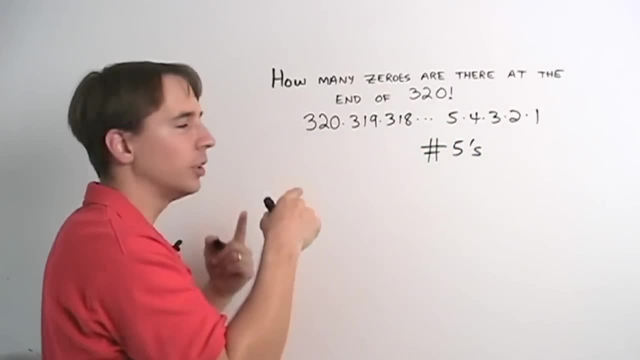 we just look at it as groups of 5,: 1 through 5,, 6 through 10,, 11 through 15, and so on. each of these groups of 5 ends in a multiple of 5.. So we have 320. 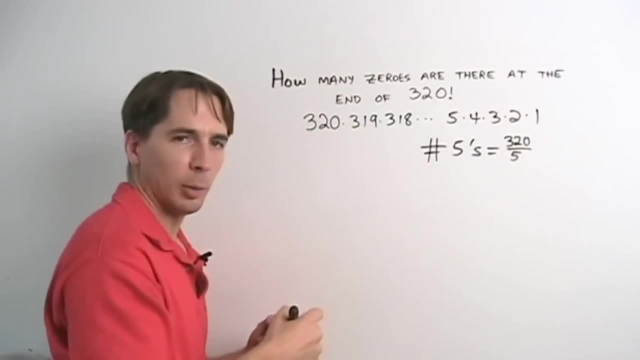 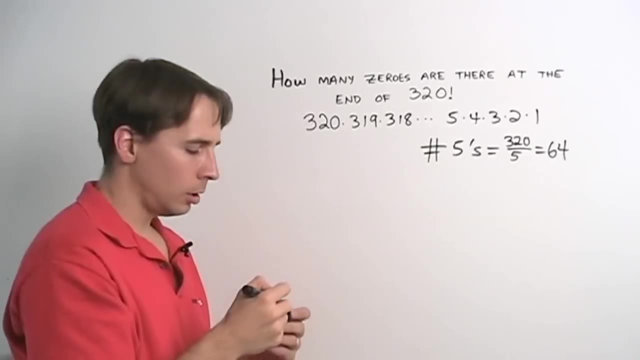 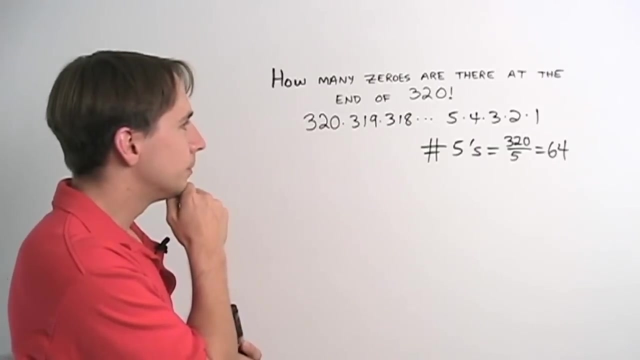 We just divide that by 5.. 300 divided by 5 is 60.. 20 divided by 5 is 4.. 60 and 4 is 64. And we see that there are 64 groups of 5 numbers here. So there are 64 multiples of 5.. Well, 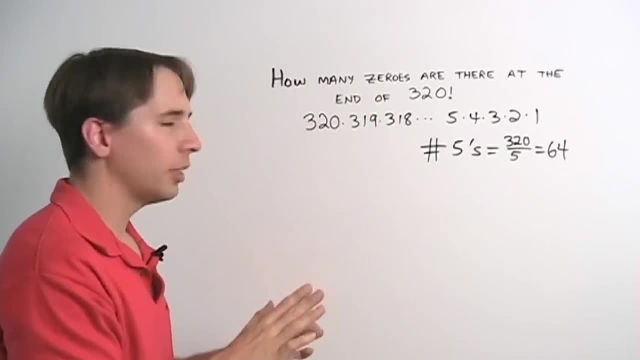 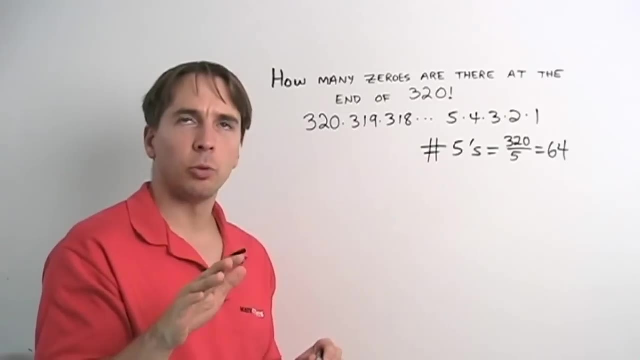 before we write down the answer and just say, OK, there are 64 zeros at the end, we should stop and think for a minute, because we already tricked ourselves once just by counting the multiples of 10.. So let's think about these multiples of 5.. Make sure we have them all. 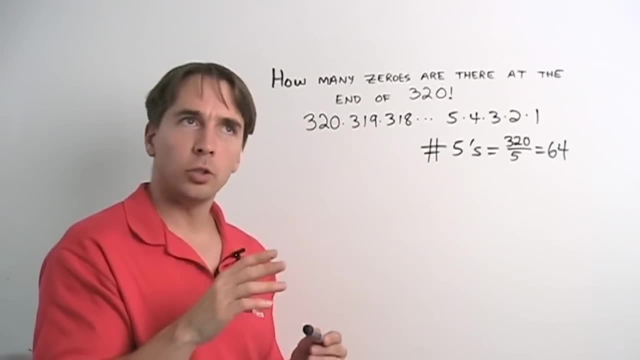 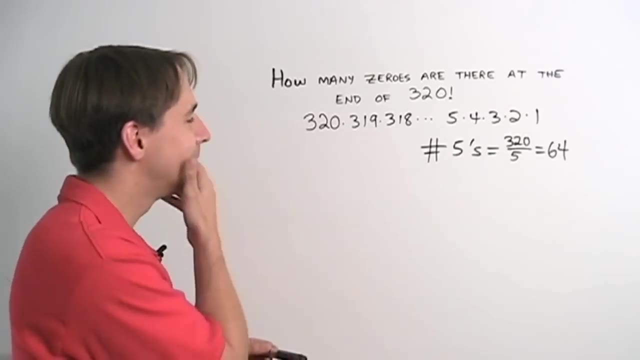 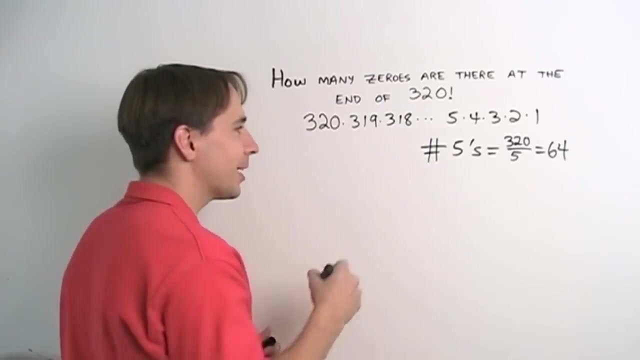 So you've got 5.. You've got 10,, 15,, 20,, 25,, oh, 25.. 25 has 2 factors of 5. Hm. So if we just count the multiples of 5, we miss those extra factors. So we have to go back and count. 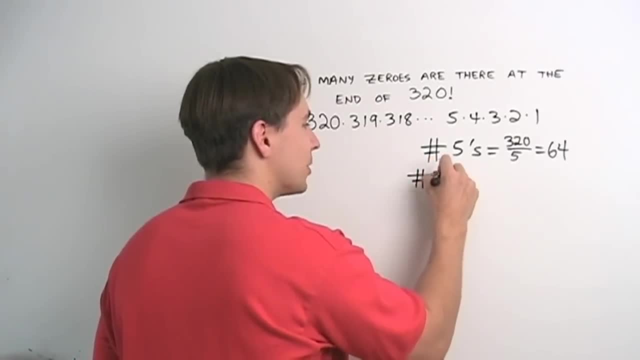 them too. We have to worry about the number of multiples of 25 in this list. Now, how many of them are there? Well, they're just 4 for each hundred: 25, 50,, 70, 500.. 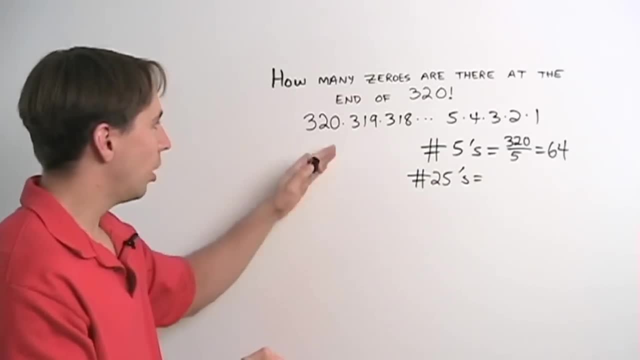 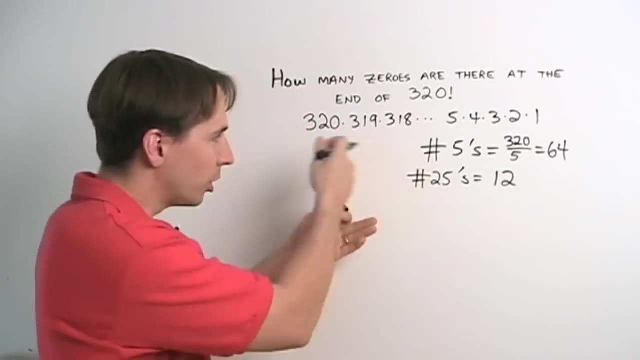 Here we go. We've got three hundreds, that gives us twelve, and the next one is three twenty-five- not in the list. so there are twelve multiples of twenty-five in this list. Well, since we had to think about the numbers with two factors of five, we should think: 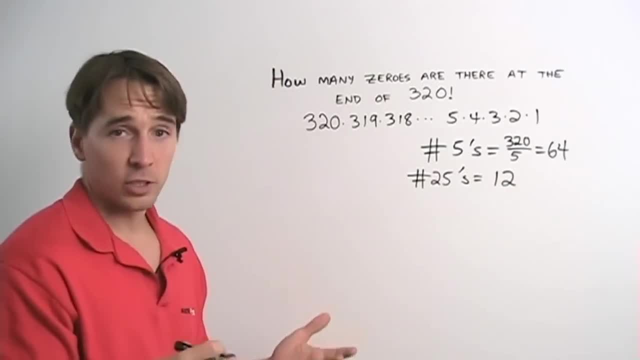 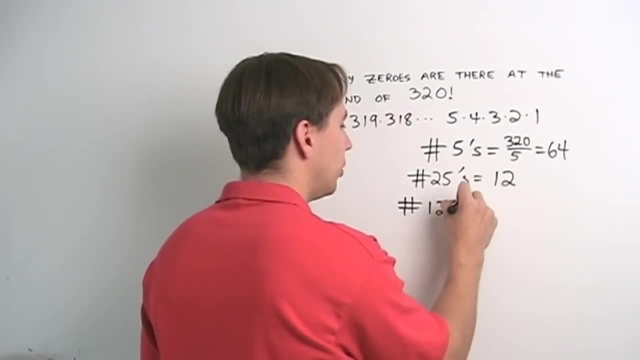 about the ones with three and four and so on. The first number with three factors of five is just five times five times five and of course that's one hundred and twenty-five. so we need to worry about the multiples of one hundred and twenty-five in this list. 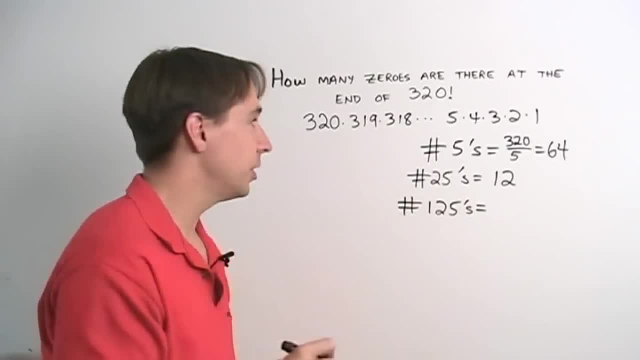 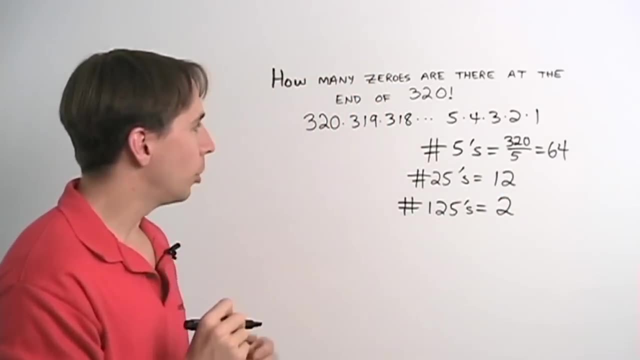 Fortunately they're easy to count. Here's one hundred and twenty-five, the next one is two fifty, the next one after that is three hundred and seventy-five, which is not in the list, and we have two multiples of one hundred and twenty-five here and then four. we have to work out four factors of. 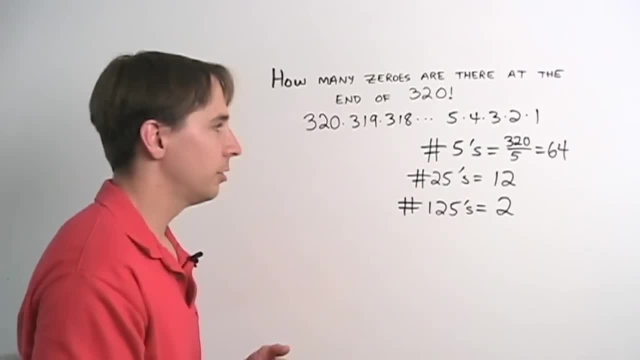 five in a single number. Well, the first one there is: five times five times five times five, that's twenty-five squared six hundred and twenty-five. that's way outside this list, so we don't have to worry about any more. 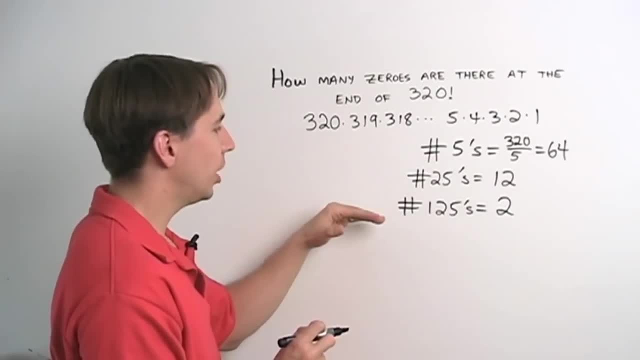 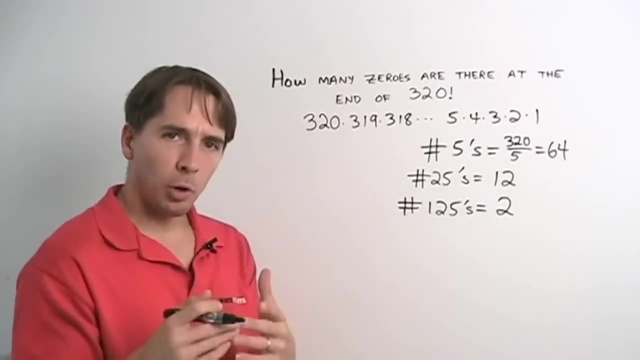 Now what do we do? We have our multiples of five, multiples of twenty-five, multiples of one hundred and twenty-five, And we want to count the number of factors here. Well, if we look at our multiples of twenty-five, we count our multiples of twenty-five once. 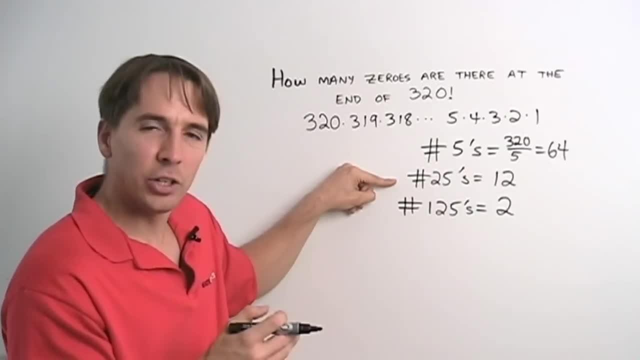 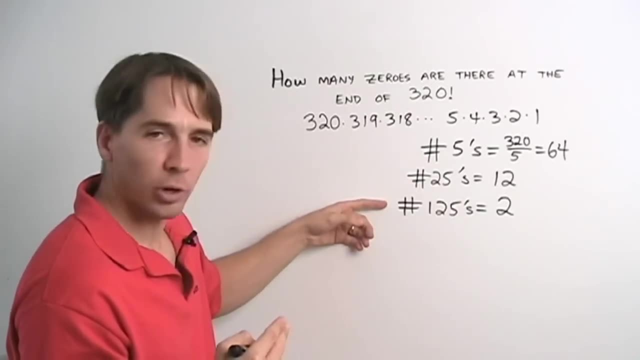 here, because they are multiples of five, and we count them again here. and that's exactly what we want to do. We want to count them twice, once for each factor of five, and a similar thing happens with our hundred and twenty-fives. 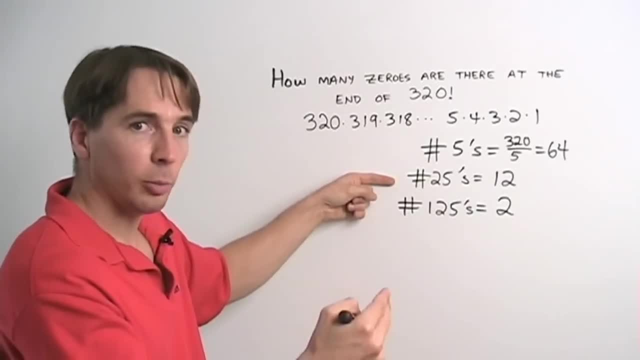 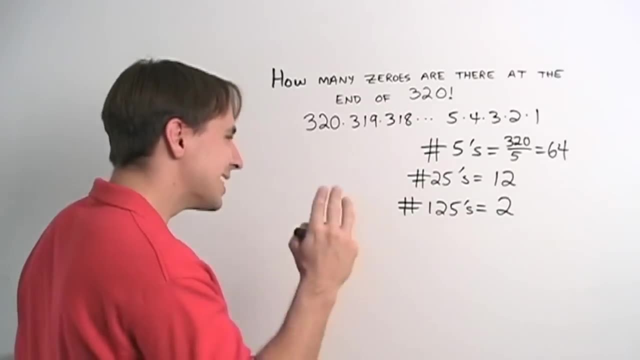 We count them once here because they're multiples of five, count them once here because they're multiples of twenty-five, and then we count them again here because they're multiples of a hundred and twenty-five. We count them three times for each factor of 5, and that's exactly what we want to do. So we see that if we just add 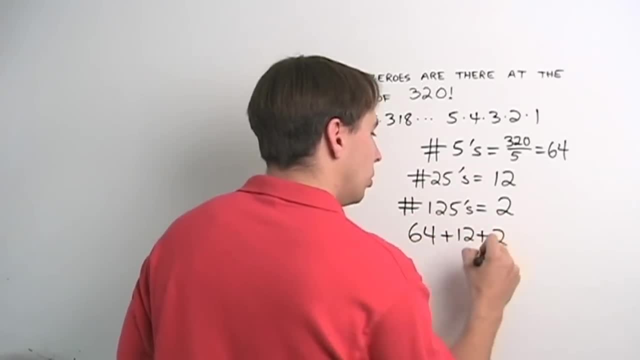 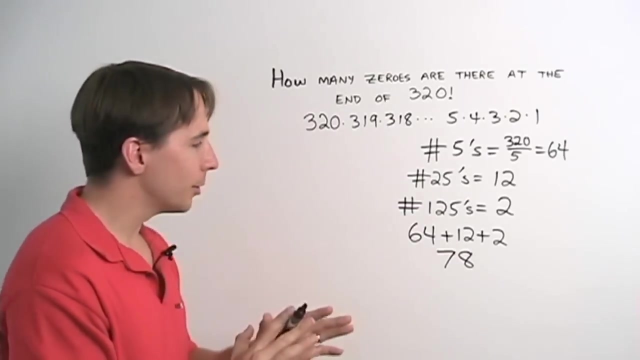 these three numbers, we get the total number of factors of 5 in 320 factorial. When we add those up, we get 78 factors of 5 in 320 factorial. Now we've tricked ourselves a couple times already, so before we scribble down 78 and move on to the next problem, we stop and 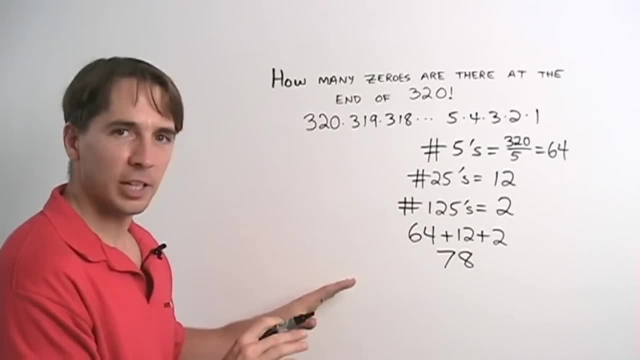 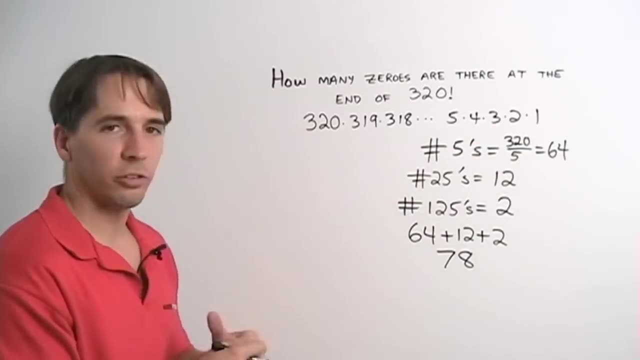 think and make sure. okay, we do have 78 factors of 5.. We're pretty confident of that. Do we have enough 2s to make the 10s? Now, fortunately we can answer that really quick. 320 numbers in the list. every other one is even so that means there are 160 even numbers. That's a 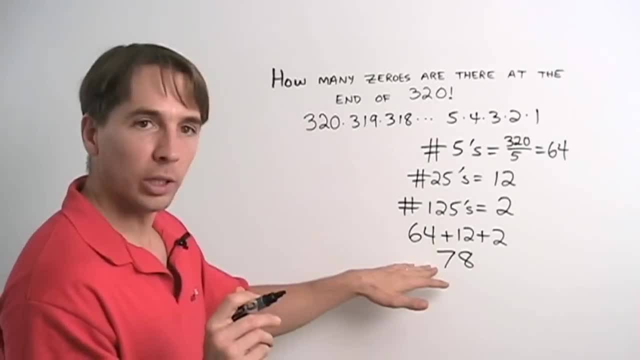 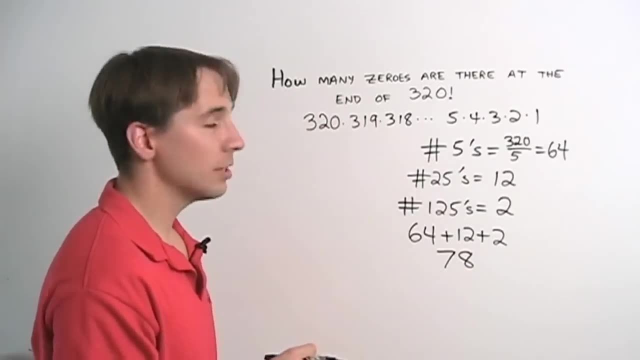 lot of 2s. It's at least 160 2s, So we can pair off enough 2s with these 78 5s to make 78 10s And 78 10s. well, 78 10s give us 78 zeros at the end of 320 factorial. 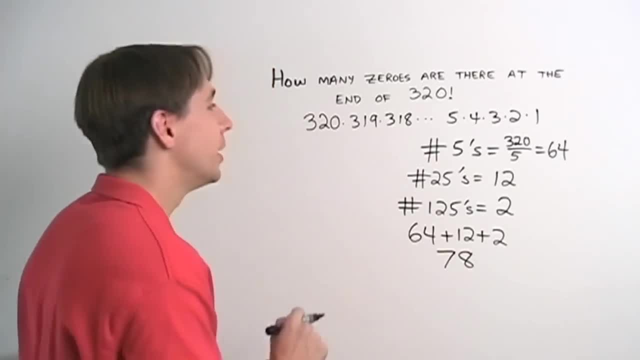 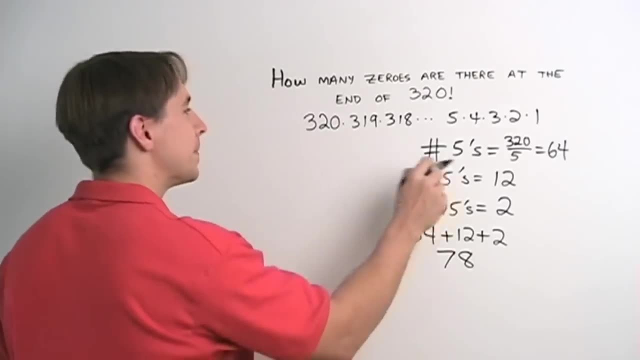 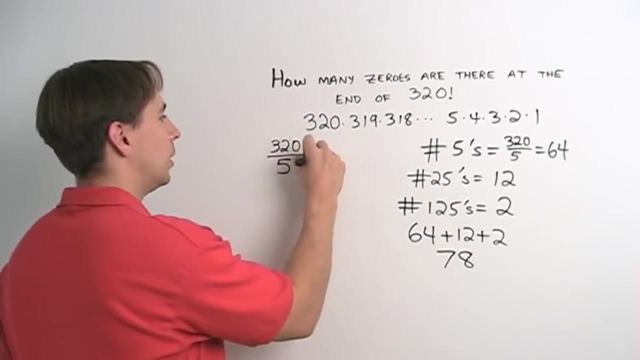 But wait, there's more, Not more, zeros. There's more to this problem. Let me show you a slicker way to do it. Take the 320 and divide by 5, and that gives us 64. Then we take this 64. 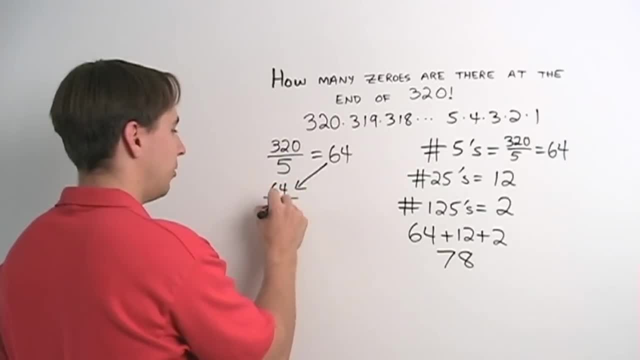 and we divide that by 5.. That gives us 12 with a remainder of 4.. And fortunately, this is one of those times when we can ignore the remainder- I like ignoring the remainder- And we take that 12 and we divide that by 5. And we get 2 with a remainder. 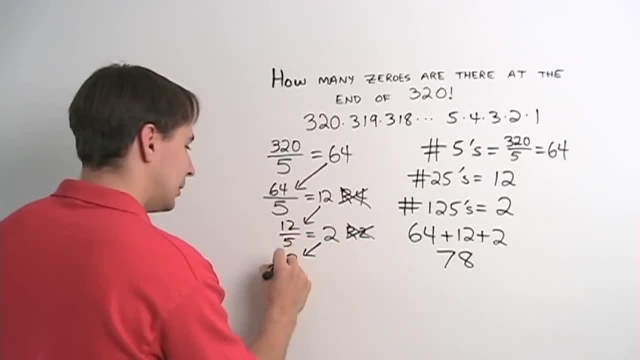 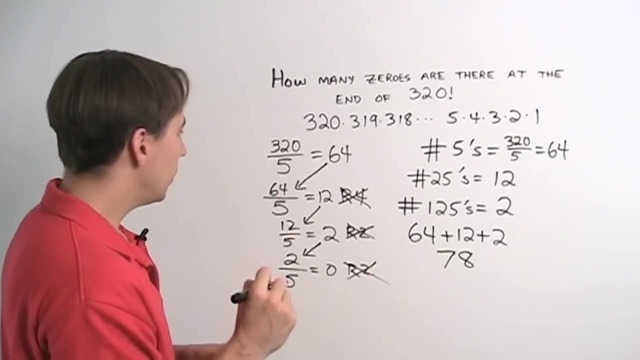 of 2, which we're going to ignore. We take 2, divide by 5, we get 0 with a remainder of 2. And that means we're done. We can ignore that remainder too. Oh, look at those numbers.